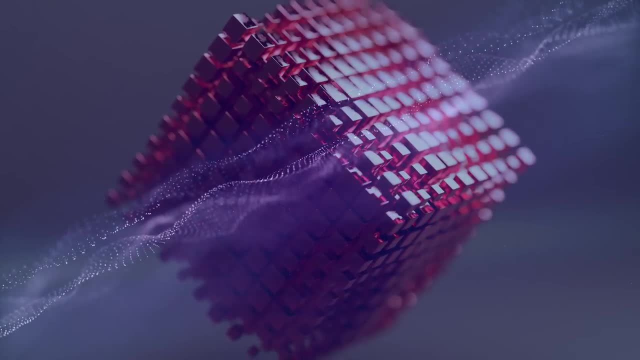 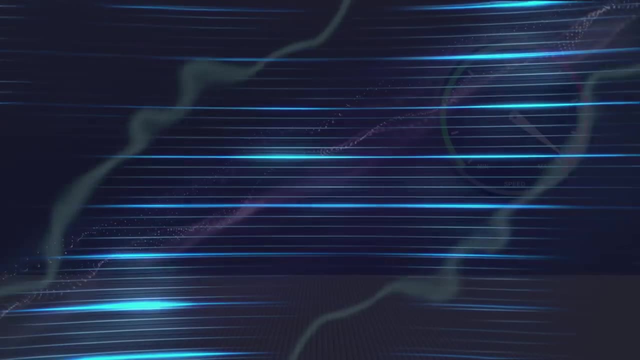 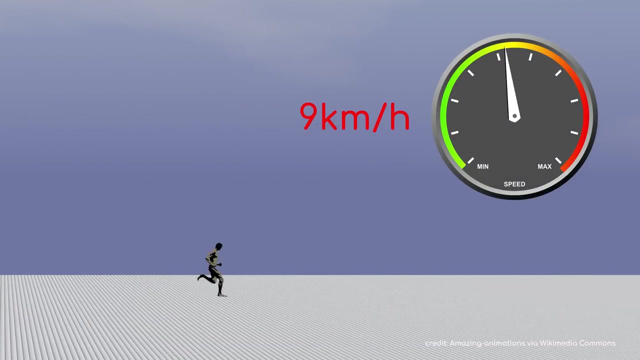 operating on one continuous scale. This is a little unintuitive, much like many things in quantum mechanics. So let's illustrate what we mean with an example. If you are running, I could ask you to half the speed you are running at. You could half your speed again, and again, and again. Is there a limit to how many times you? 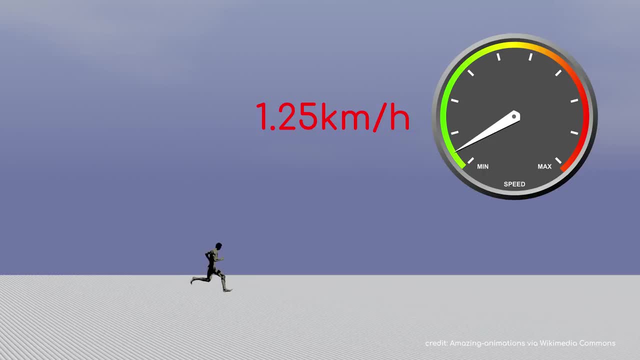 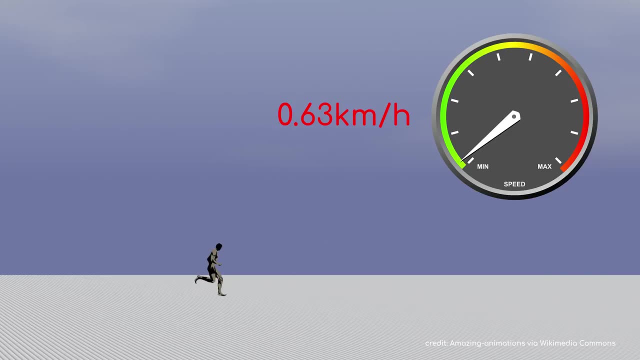 can half that speed. While you might struggle with the precision necessary to do it in classical physics, there's no reason you couldn't keep halving and halving your speed indefinitely, as there's no limit to the number of times you can divide a number by two. 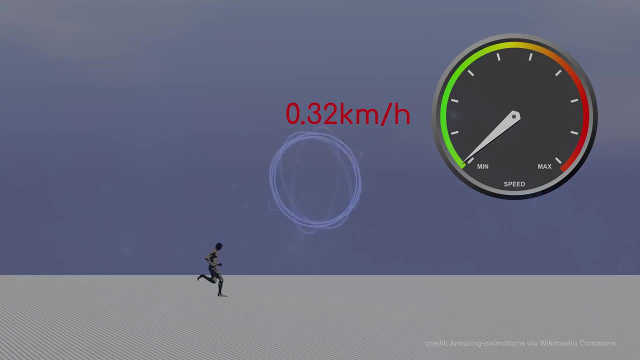 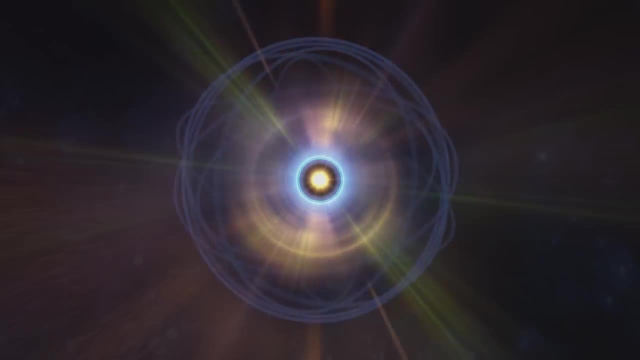 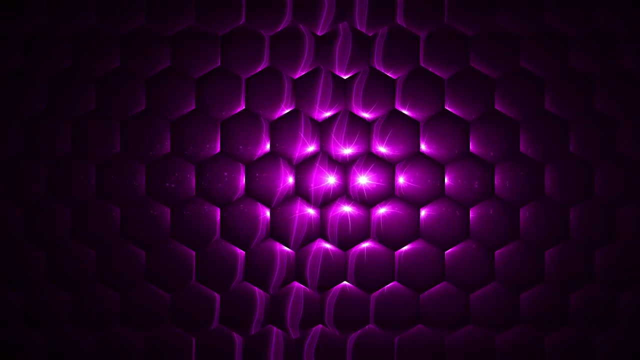 There's always a smaller number In the quantum world. this is not so When it comes to energy levels, momentum and other attributes. when you reach a small enough number, you discover that the universe does not work on a continuous scale, but rather in. 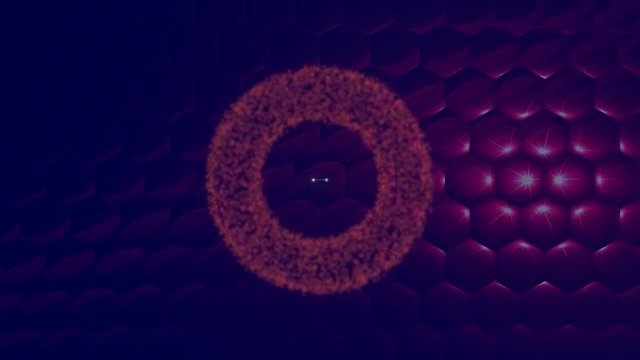 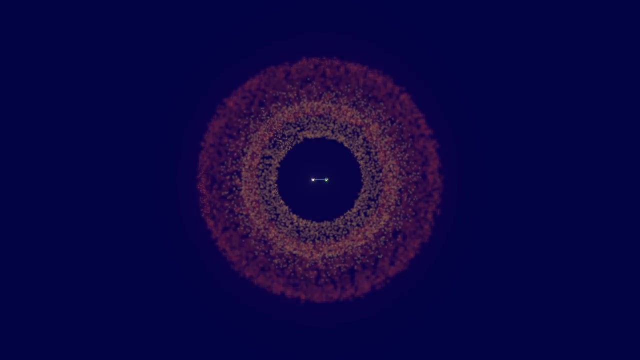 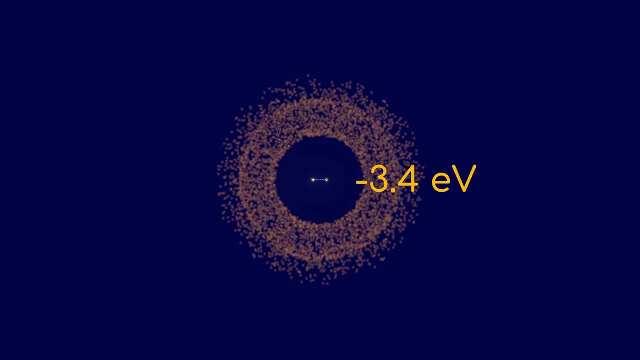 quantities. An electron in a hydrogen atom can have exactly minus 13.6. Electron volts of energy, or it can have minus 3.4 electron volts, but under no circumstance can it have an energy level between those values. This has been proven experimentally. A theory: 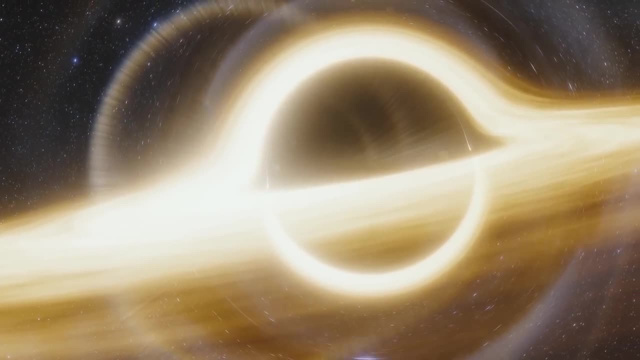 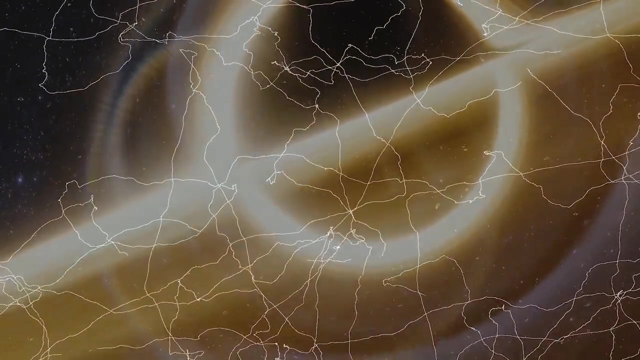 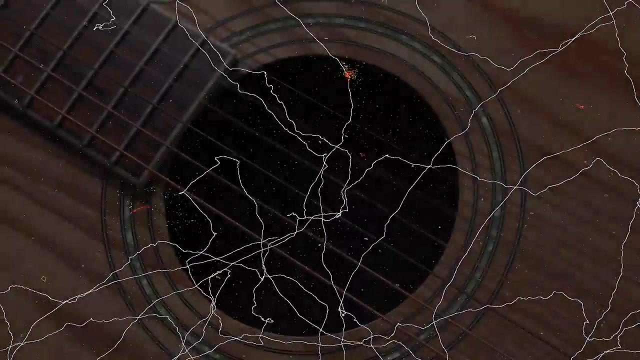 of everything must make use of an underlying universe, geometry that is fundamentally quantized. The concept of some kind of web of strings fits that bill well, particularly when you bring in the transverse. When plucking a guitar string, a standing wave can form that has one peak or two, but not a value. 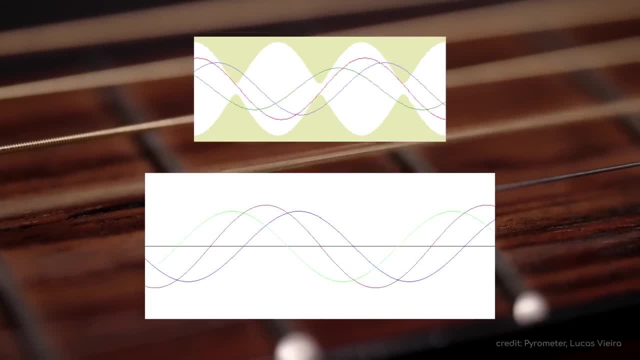 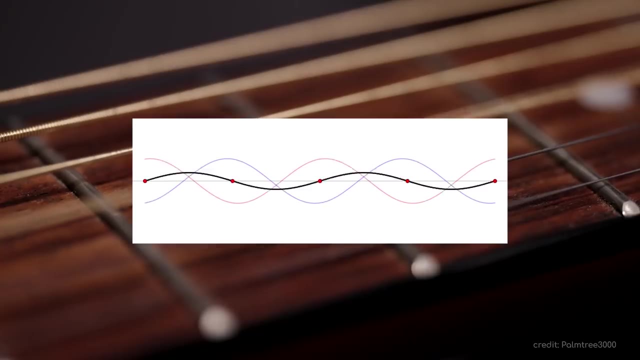 in between those. This is because harmonics are formed by a combination of waves travelling along the string in one direction, perfectly resonating with waves travelling in the other. If the speed or frequency of the waves don't line up perfectly, the two waves will ultimately disrupt each other. 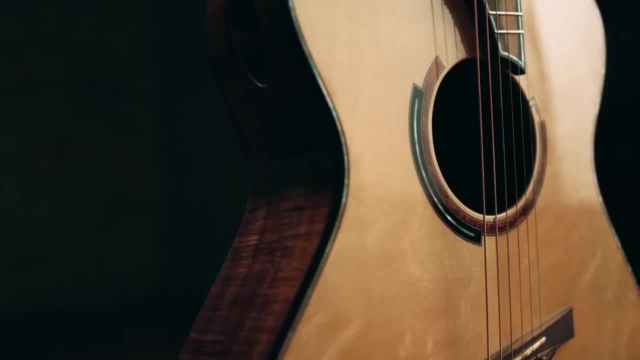 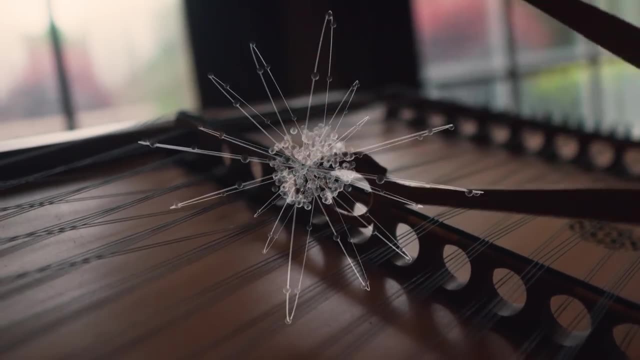 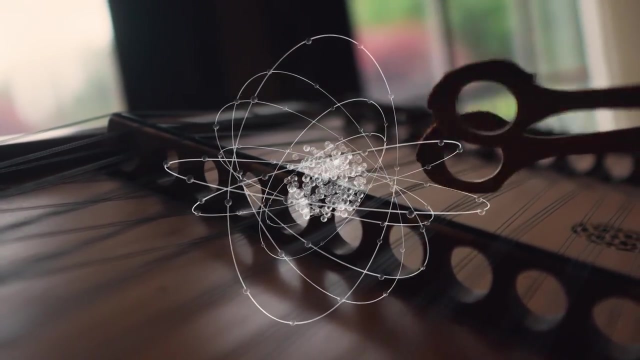 leading to the collapse of the standing wave. Only waves with just the right amount of speed and energy can create standing waves on a given string. So immediately we have an interesting mirror to our observation that subatomic particles have quantized momenta and energy levels. So do standing waves on strings. 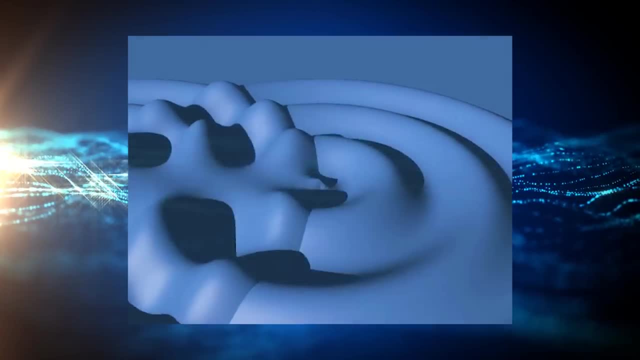 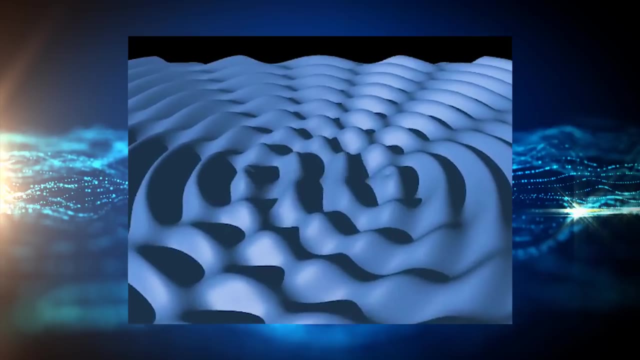 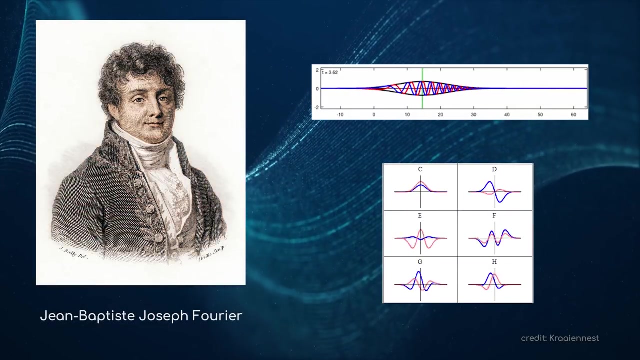 The next interesting point to note about waves is that by combining the correct sequence of sine waves, you can create any wave pattern of wave you might desire. This is a very useful principle, handy for creating the rich complexity of a universe. This mathematical principle was first discovered by Jean-Baptiste Joseph Fourier, a French mathematician. 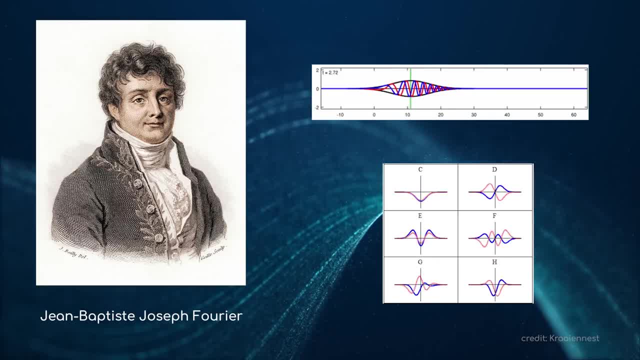 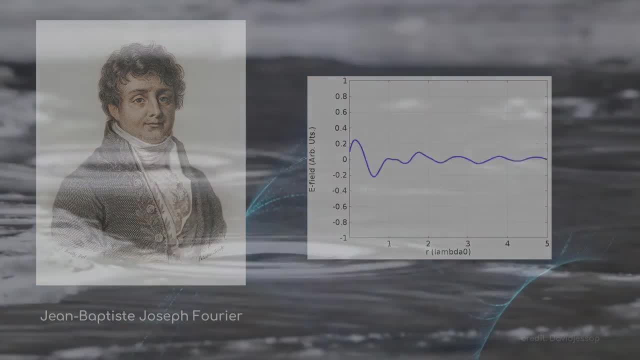 and is very useful in the study of heat transfer and vibrations, as it works the other way too. Any wave can be broken down into a number of constituent sine waves. When two waves try to occupy the same place, they will amplify each other if they are both rising or 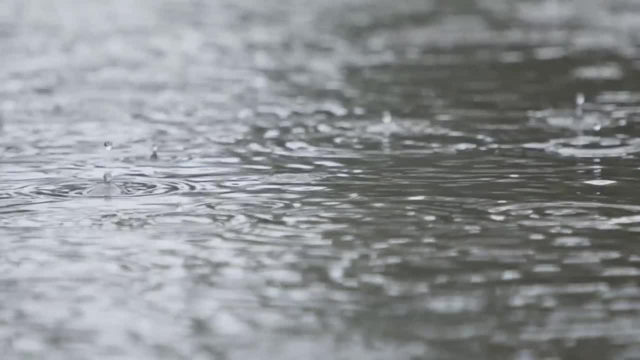 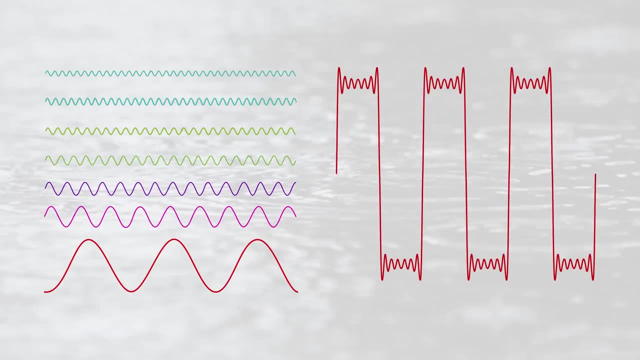 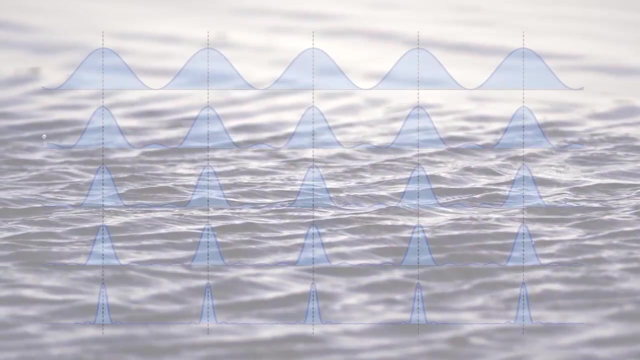 both falling but will cancel each other out if they are in opposition. This can lead to all sorts of waves being formed: square waves, intermittent waves and even waves that only have a single peak and are flat at all other locations. This becomes easier to do the more waves you have to overlap. 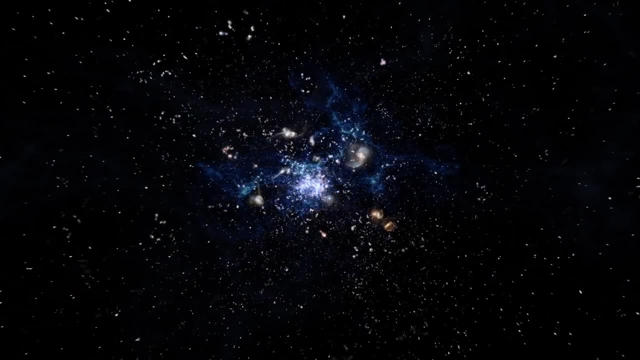 This is an interesting observation as it helps answer an important question: that any theory of everything must be able to answer. This is an interesting observation as it helps answer an important question: that any theory of everything must be able to answer. This is an interesting observation as it helps answer an important question: that any theory of everything must be able to answer. 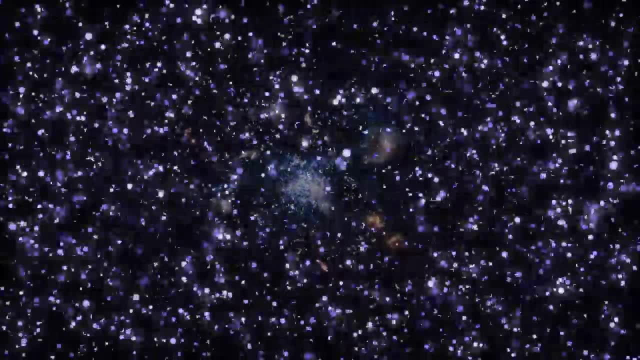 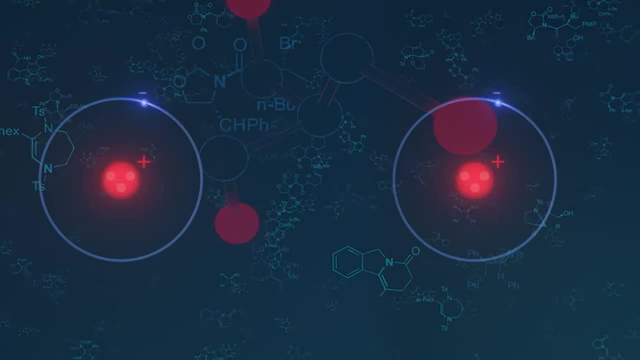 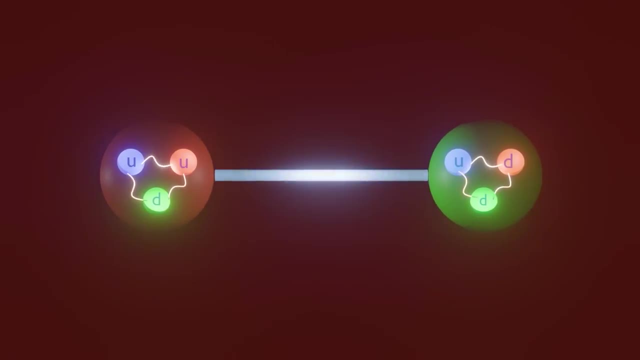 Where do particles come from? When I say particles, I'm not specifically talking about molecules or atoms, but the components that make these objects up. Atoms split into protons, neutrons and electrons. Protons and neutrons split into quarks, and there are leptons and bosons. 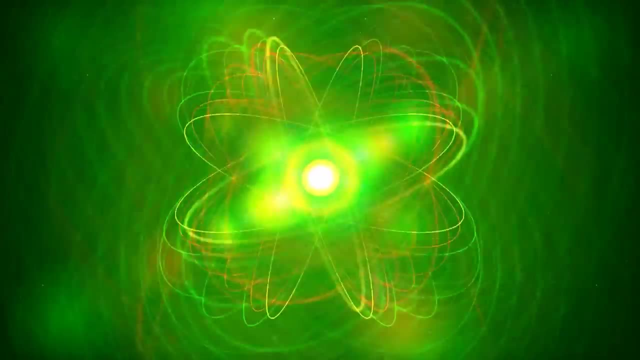 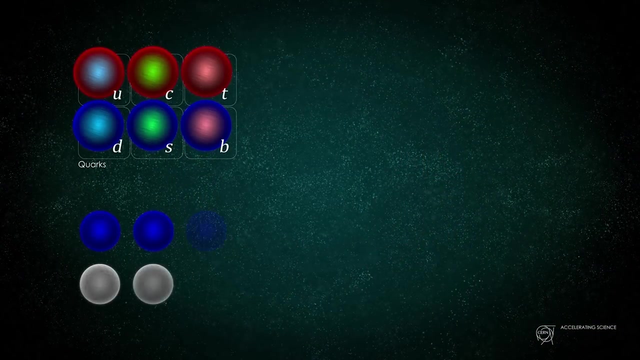 Without needing to go into exactly what all of these things are or why they have some of the weird names that they do. I mean, who'd decide? I mean who'd decide? It's enough to say that they come in many different flavours. 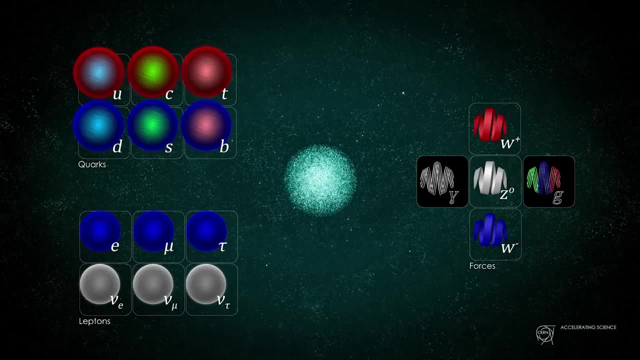 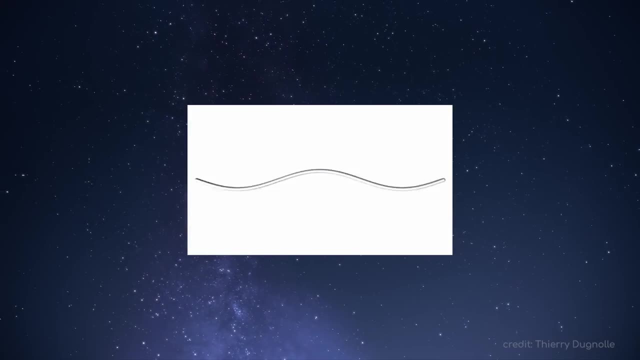 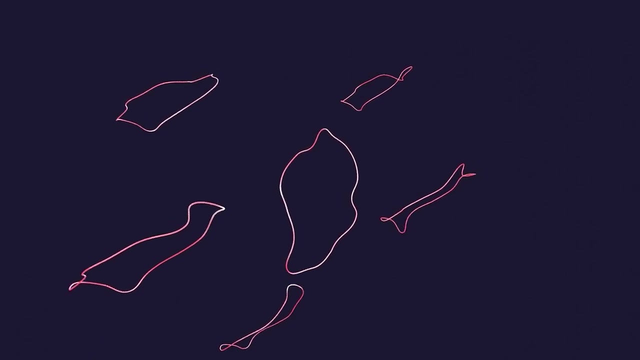 These are the smallest building blocks of reality that we know of so far. Why do they exist? Well, in a model using strings, they are the rising and falling of a wave. This matches Einstein's observation that mass and energy were essentially just the same thing in different forms. 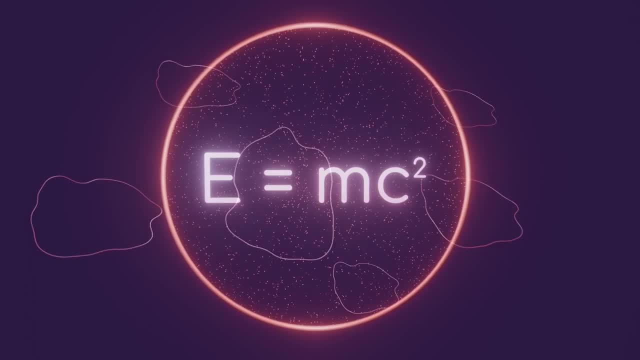 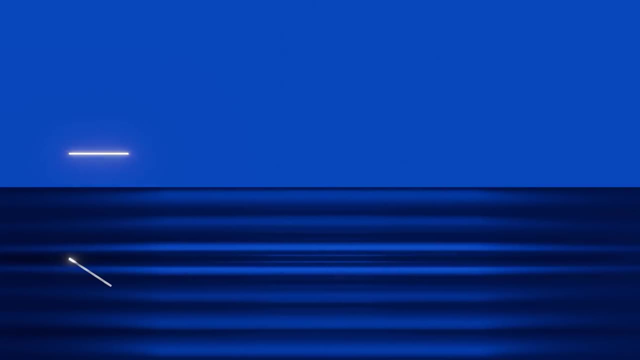 This matches Einstein's observation that mass and energy were essentially just the same thing in different forms, which he found out in his E equals mc squared equation. A wave is the motion of energy. Mass can be that too. The narrower the peak of the wave, the more defined a particle is in terms of its location on that string. 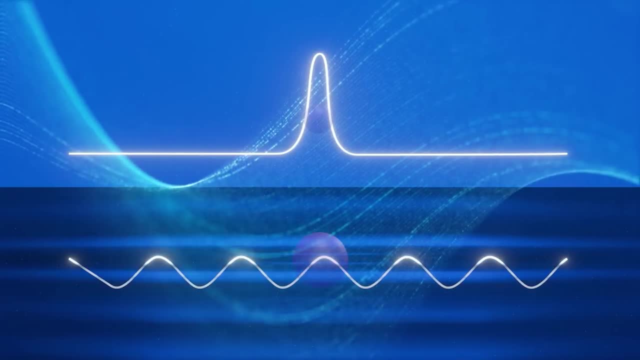 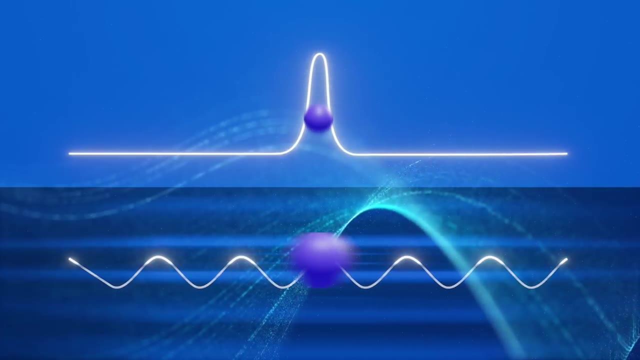 You might take issue with the idea that both of these waves represent the location of a single particle. However, curiously, this matches another important facet of particles. However curiously, this matches another important facet of particles: Where exactly they are in space. 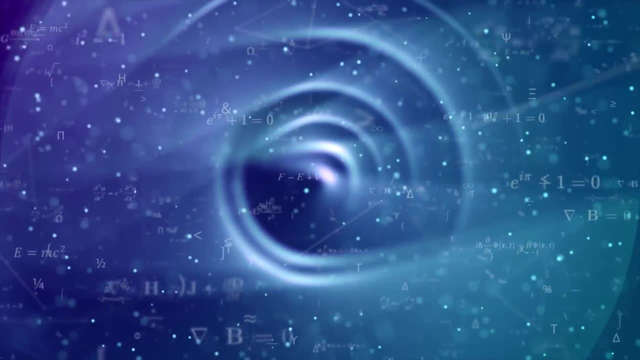 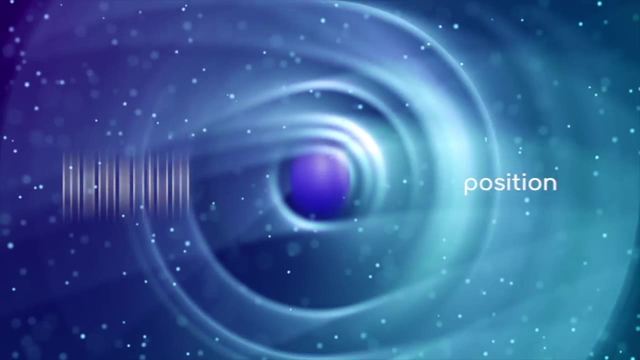 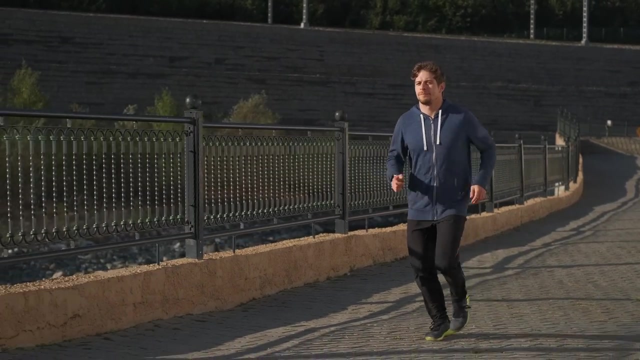 If you know much about quantum mechanics, you have likely heard of Heisenberg's uncertainty principle. This is the idea that we cannot know a particle's momentum and position at the same time. We get a decent approximation at large scales. It's pretty easy to see where you are and where you're going. 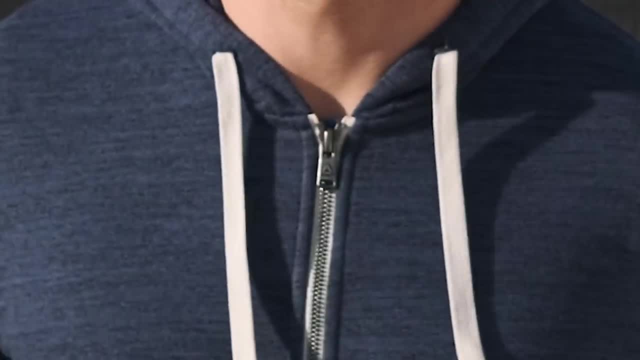 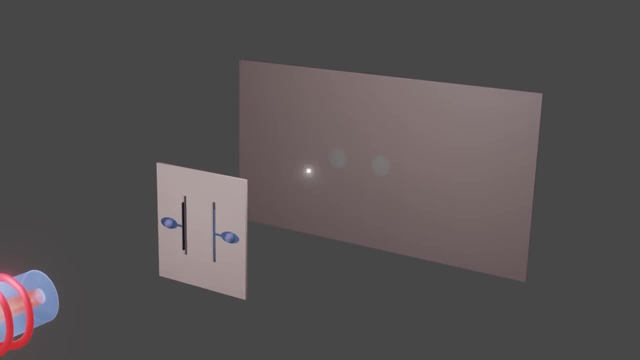 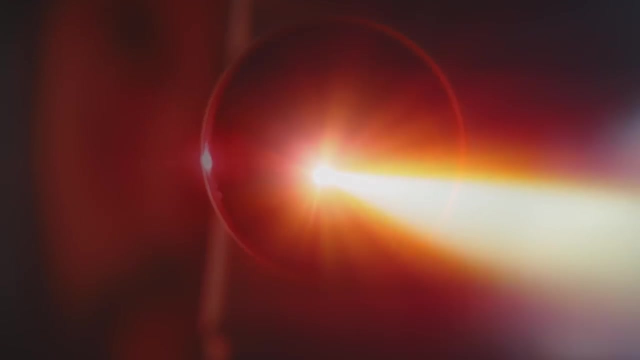 But at small enough levels, this becomes impossible to do. The more precisely we know where a photon is, the less information we have about its momentum, And vice versa. This isn't just because we have bad techniques for observing them. This is apparently a fundamental truth. 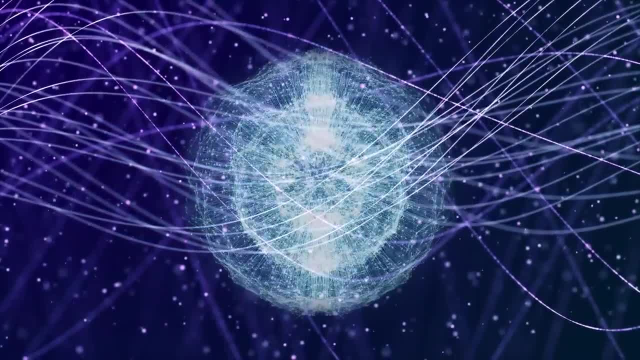 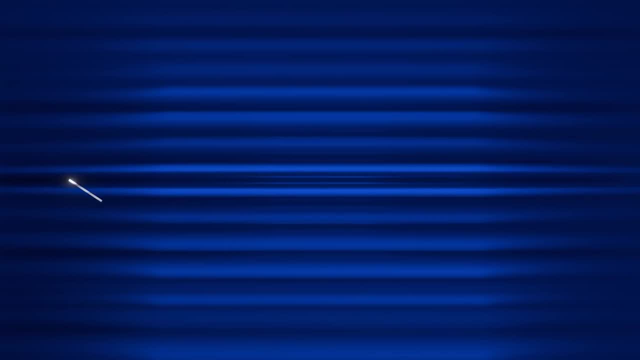 If we think about particles being the sum of many overlapping waves, however, this suddenly makes a lot more sense. Take a look at this wave. It is perfectly defined in terms of where it is going, but if we consider the peaks of this wave to represent the location of the subatomic particle? 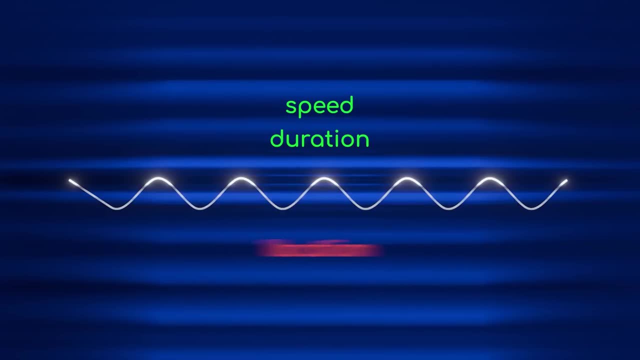 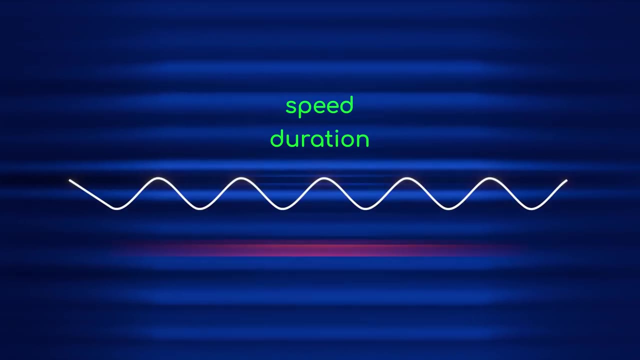 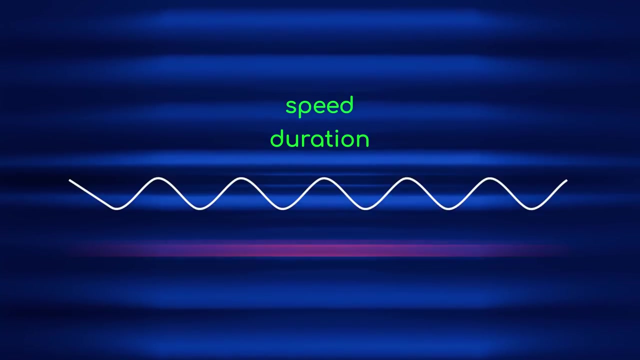 or at least the possibility that the particle is at this location. there are a lot of places it can be. So for this given string, we have perfect knowledge as to its speed and direction, but are uncertain about its position in a given space of string. 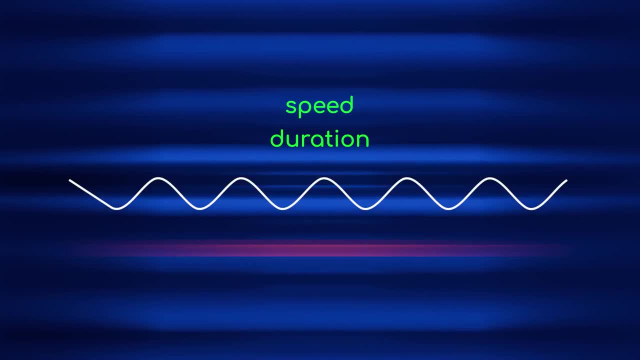 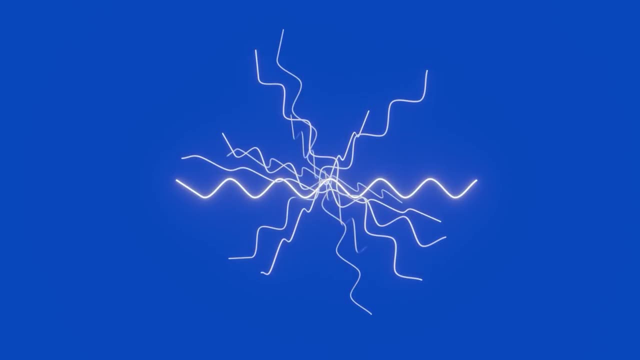 perfectly in line with Heisenberg's uncertainty principle. If we converge several different waves into a single point, we can take advantage of Fourier's mathematical tricks to cancel out some of the peaks of our wave, The more waves we add coming in from different directions. 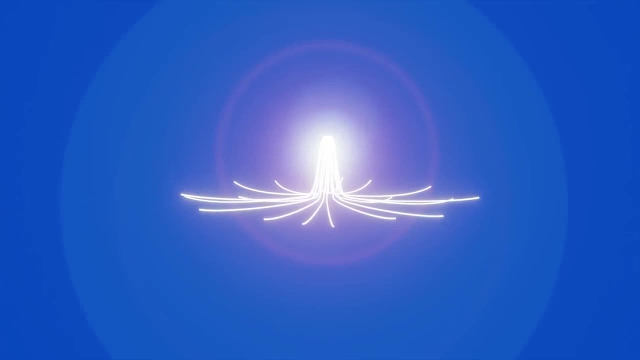 the more our particle becomes defined in space. But look at our particle now. How many strings are running through it? Each of these is a separate vector line representing momentum in a different direction. It's no longer quite so possible to pin down where this particle is going next. 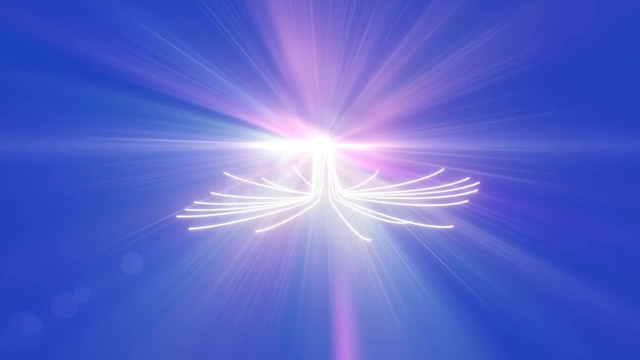 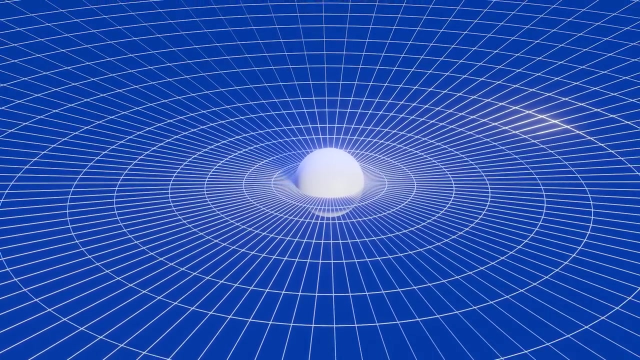 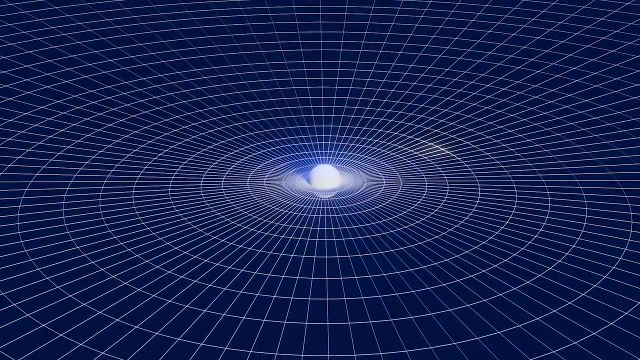 as there are several options that could be true. Perfectly pinning down a particle in terms of its location would require vector lines that could lead anywhere. This is starting to get into territory where you would need information from the entire universe before a single particle can be truly solved in terms of its location in space and time. 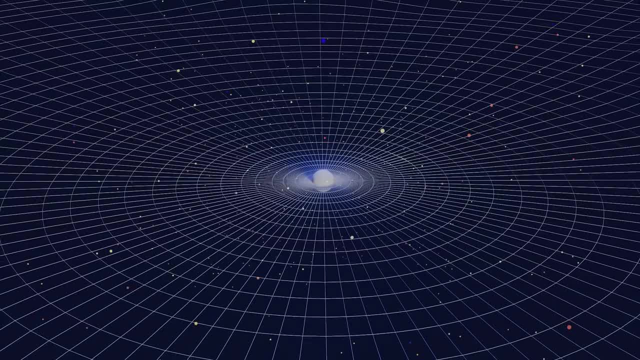 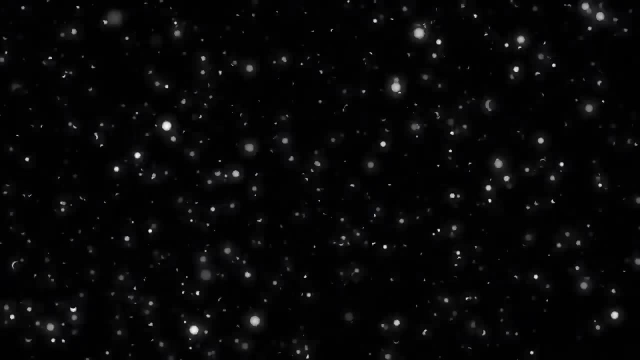 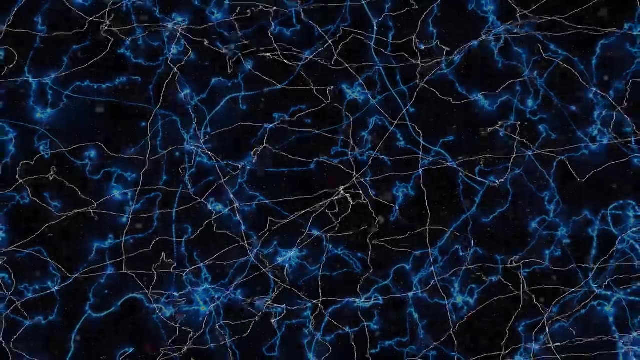 which is a little headache-inducing. Perhaps the universe makes do with close approximations most of the time until someone looks closely For this model. we must discard our concept of a particle as a localised object, but instead we define them as the convergence of different waves. 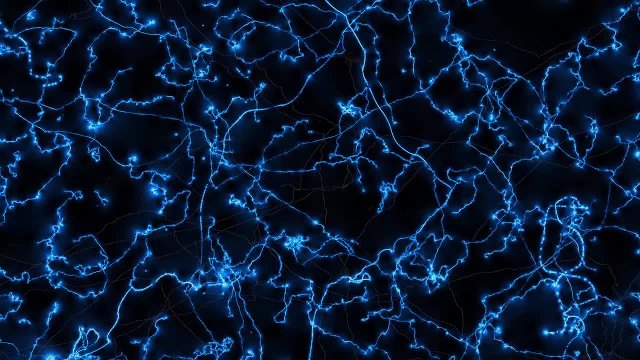 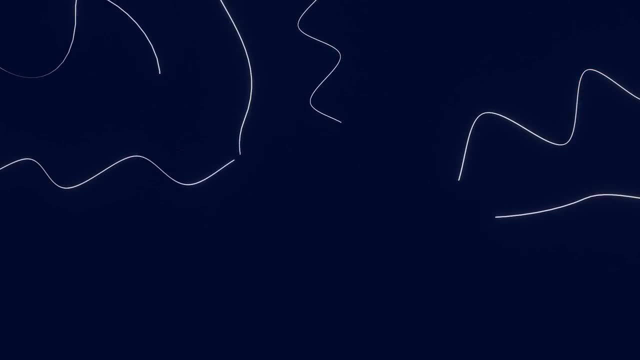 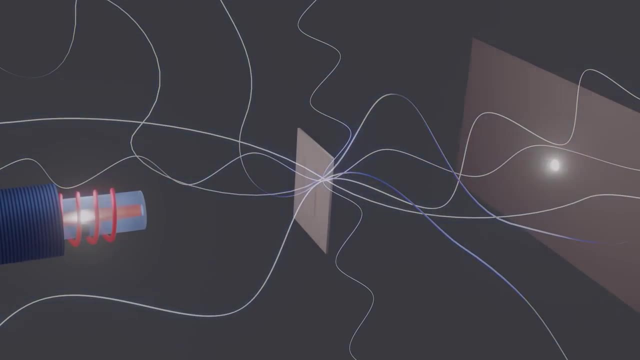 coming together at a single point and then diverging again. This divergence doesn't feel right to us. We are uncomfortable with the idea of our particles only being really there at a given moment and dissipating afterwards. However, those of you familiar with the double slit experiment, 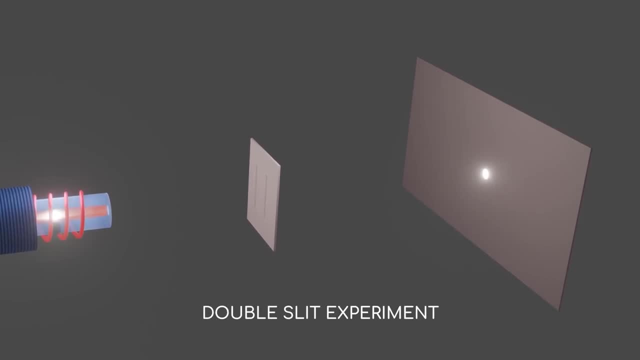 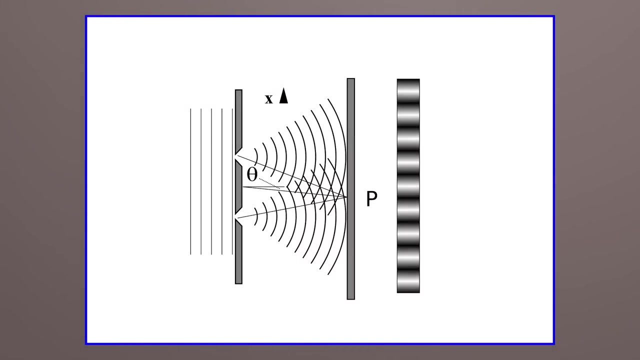 which I have covered in an earlier video, recognise that this is an uncanny match to another odd experimental result. A single photon released from an emitter and passing through two slits will somehow pass through both slits, interfering with itself on its journey. 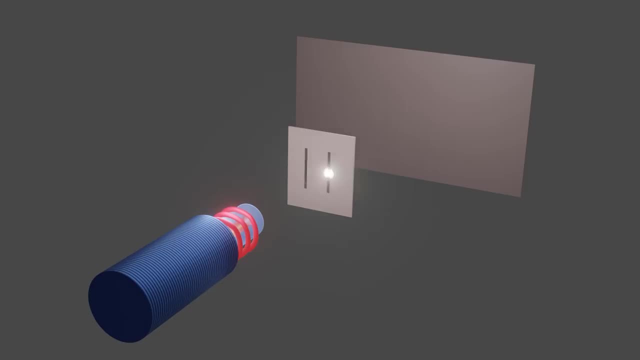 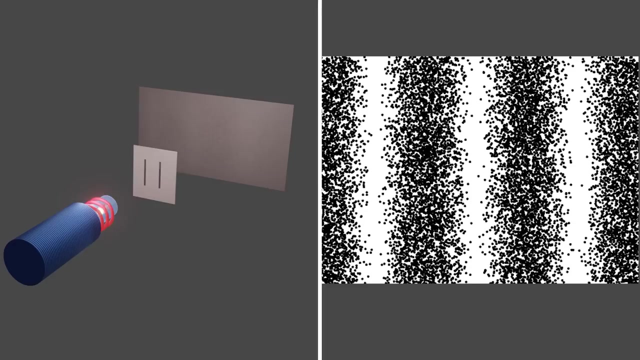 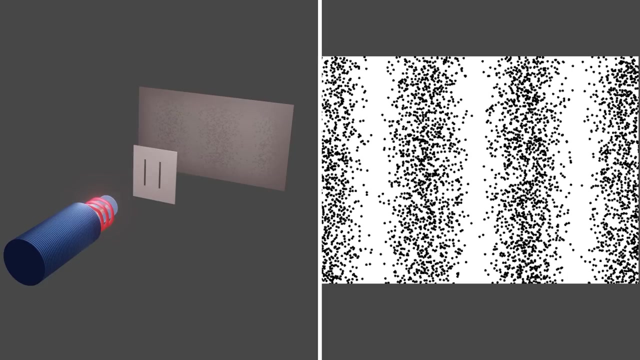 The photon reaches the far detector as a single particle, again indicating a new convergence at that point. but by sending many photons along this path, it becomes clear that interference is taking place in the intervening space. The photon seems to leave as a particle. 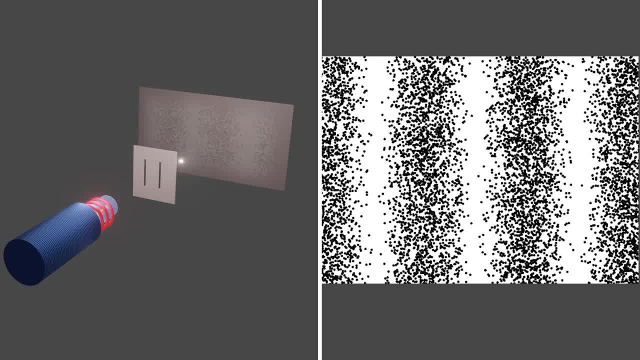 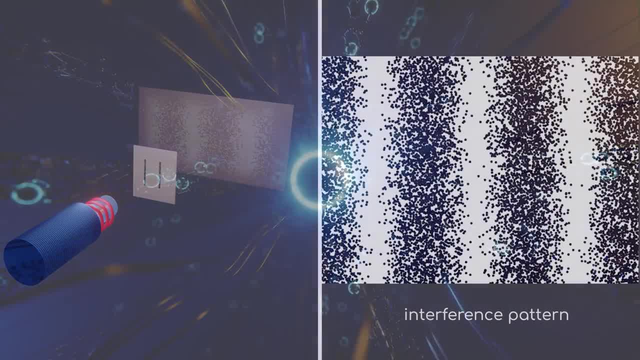 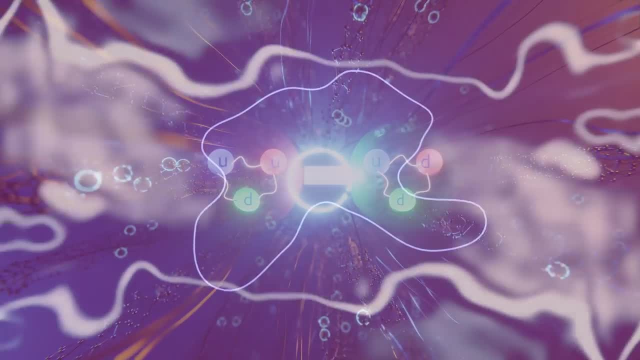 and arrive as a particle, but in the intervening space it takes on the properties of a propagating rippling wave. Already we begin to see how some of the strangest aspects of the quantum world fit with the idea of strings carrying waves of energy. 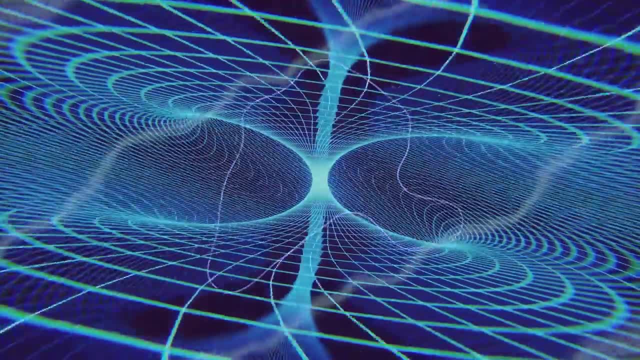 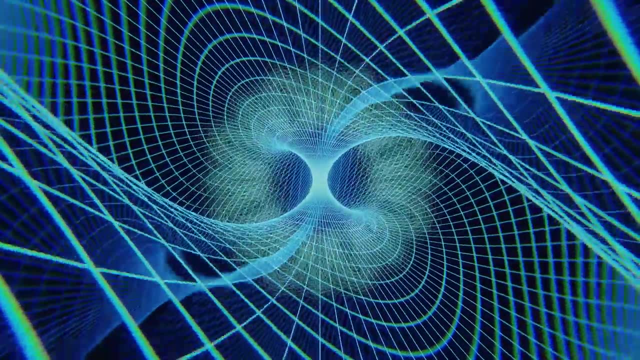 But this is only the first part of my model. To really see how much a theory matters and how it matches the universe around us, we need to explore the motion of particles across time and space to better understand entanglement and superpositions. 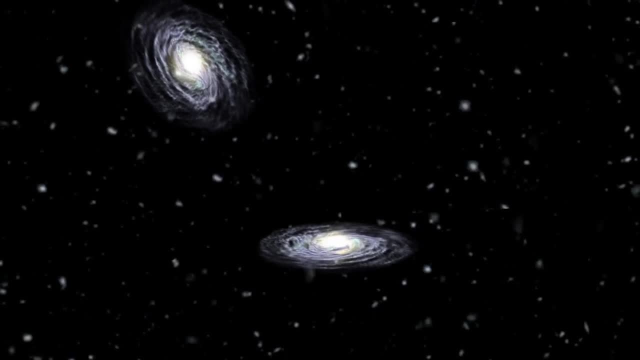 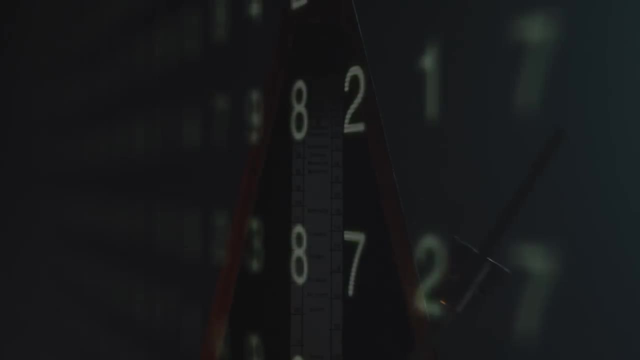 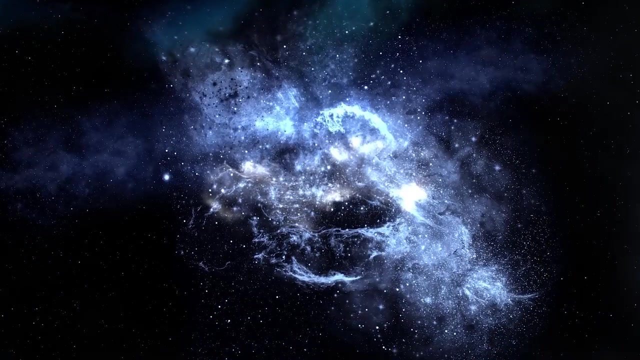 and to do that we need to explore how strings lead to gravity, time dilation and other principles of relativity on larger scales. We need to have a clear concept of how time works. My model accommodates that, but it will have to wait until my third video in this series.